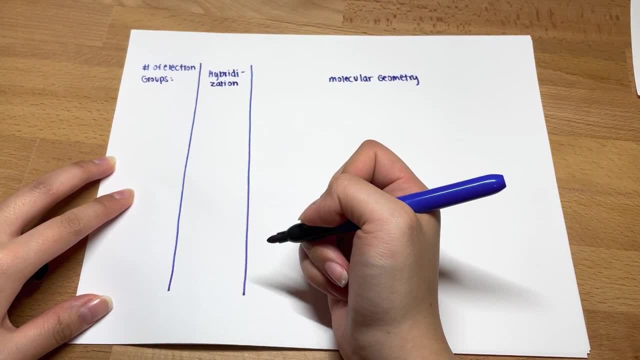 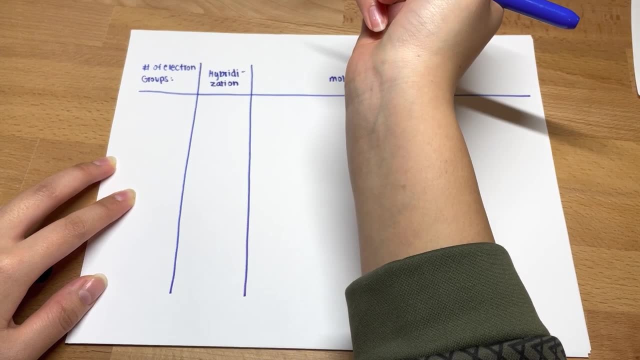 Is this columns or rows? You want to draw columns? yes, And then here we go. List all of the uh number of electron groups. So there's two, three, four, five, six, seven, eight, nine, ten, eleven, twelve, thirteen, fourteen, fifteen, sixteen, sixteen. 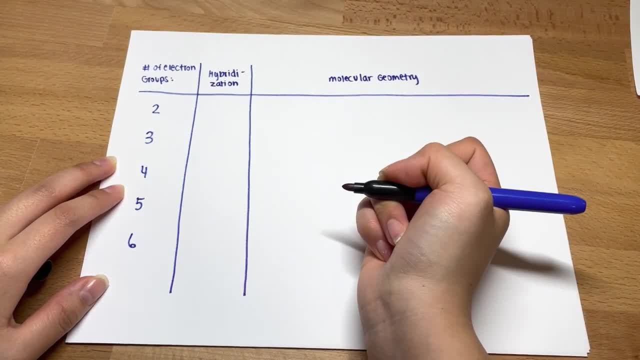 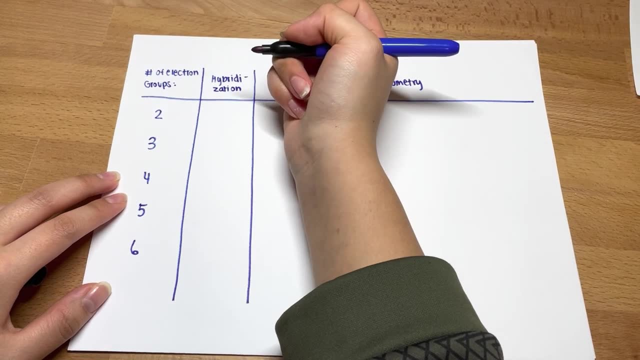 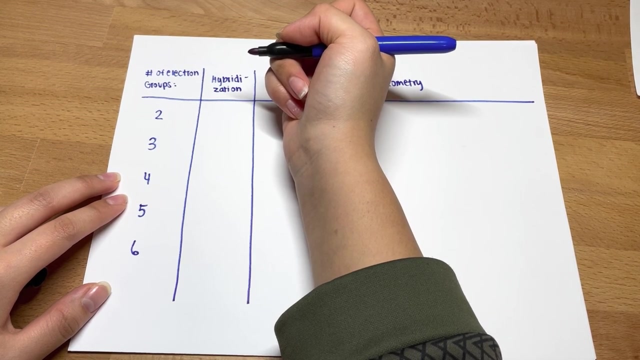 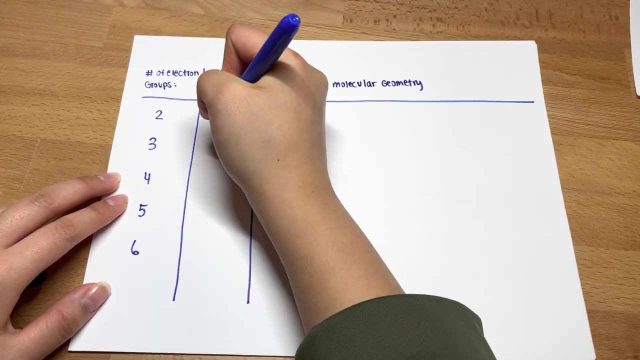 twenty, twenty-two, twenty-three, twenty-four, twenty-five, twenty-six, Okay, now hybridization. Remember, imagine: for every letter without a superscript you want to imagine, there's an imaginary one. So, sp. there's one here, one here. one plus one is two. Okay, sp. two. one here, two here. one plus two is three. 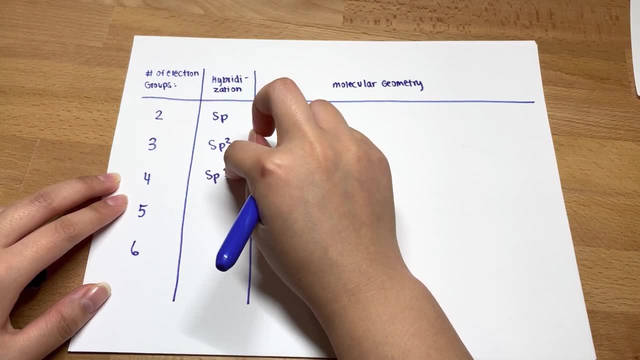 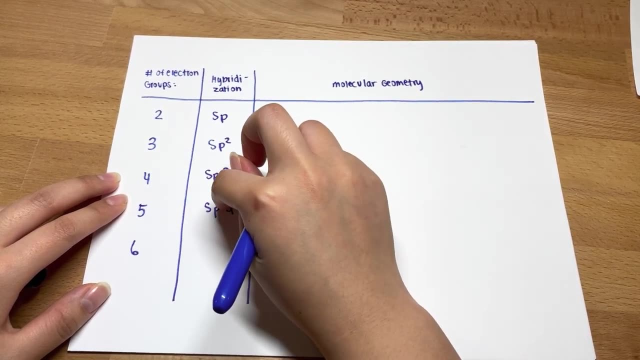 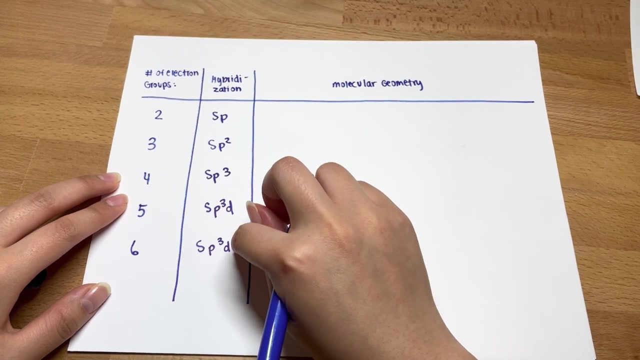 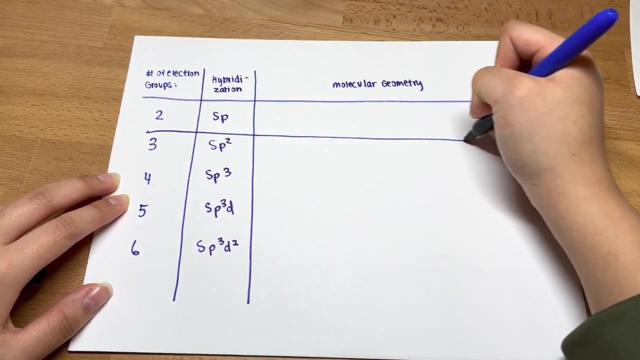 sp three: one here, three here. three plus one is four. sp three d three: one. one. three plus two is five. sp three: d two, three, four, five, six, which is six. Okay, Now you want to draw more rows, because this is how you were gonna. 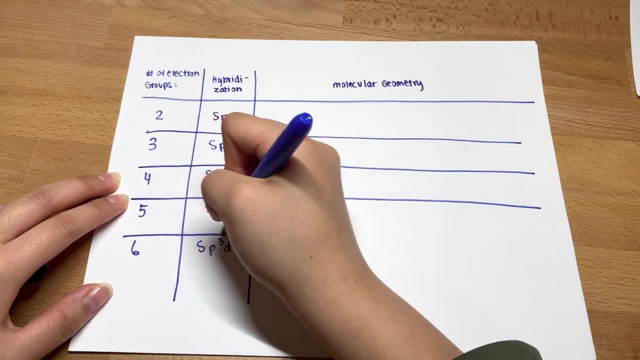 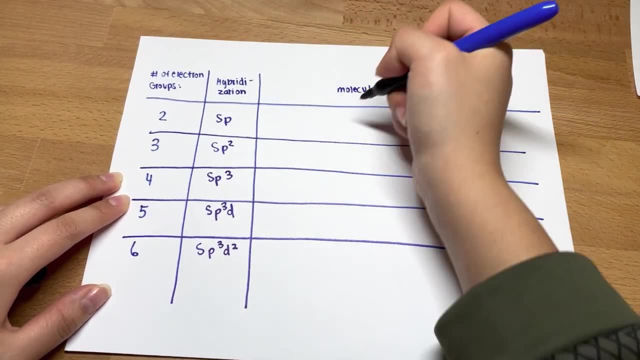 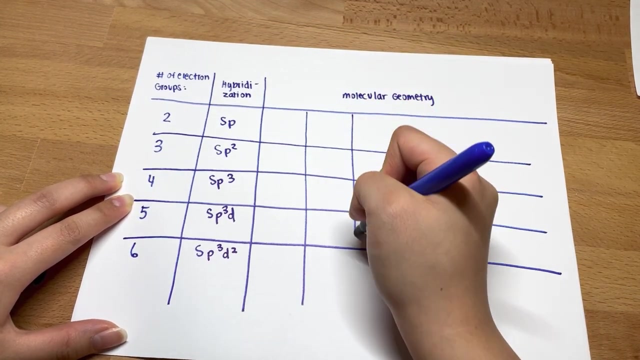 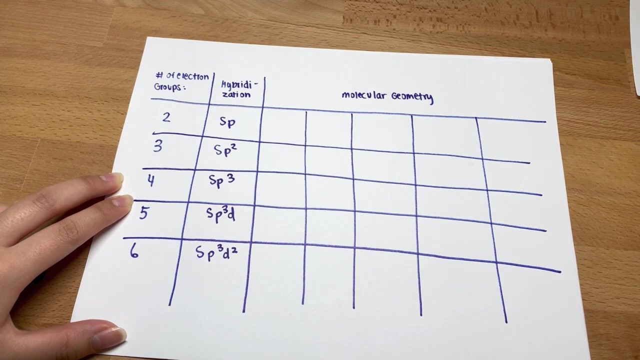 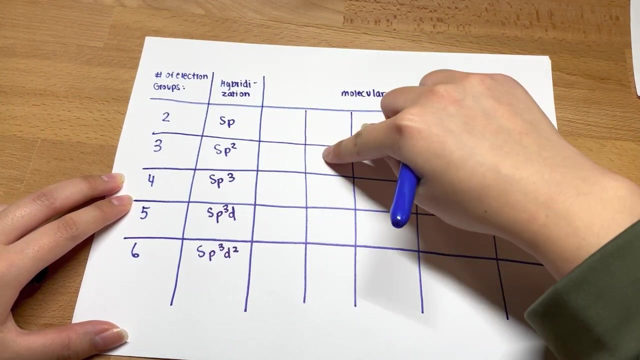 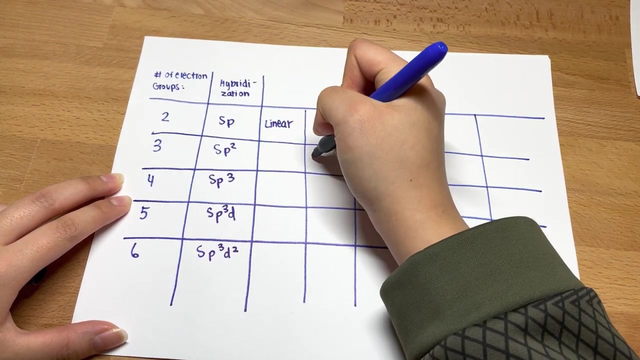 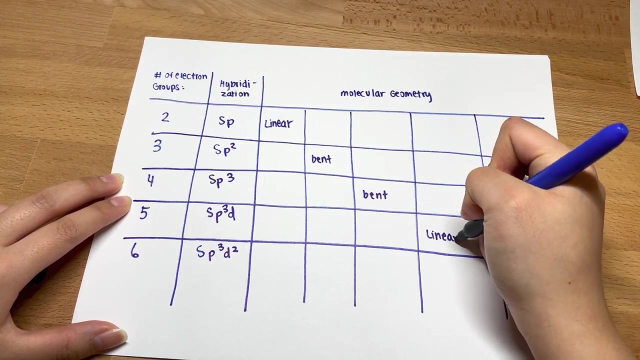 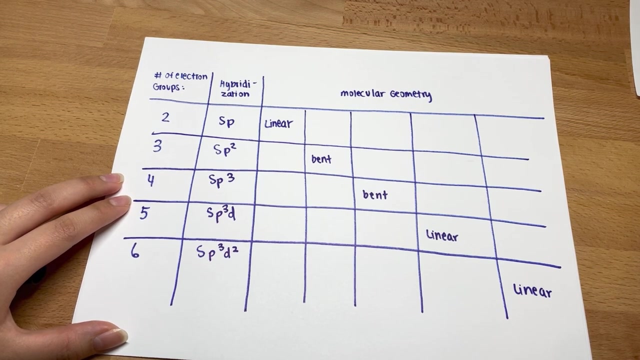 differentiate between each electron. okay, now that you have this, you want to make five columns, so draw one, two, three, four, five. like this: one, two, three, four, five. after that, here is how you're gonna remember the molecular geometry, okay, linear, bent, bent, linear, linear, easy linear, bent, bent, linear, linear. okay, now, if you can remember the electron group geometry, it would. 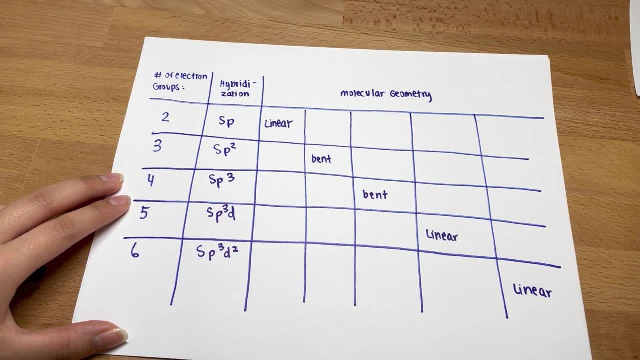 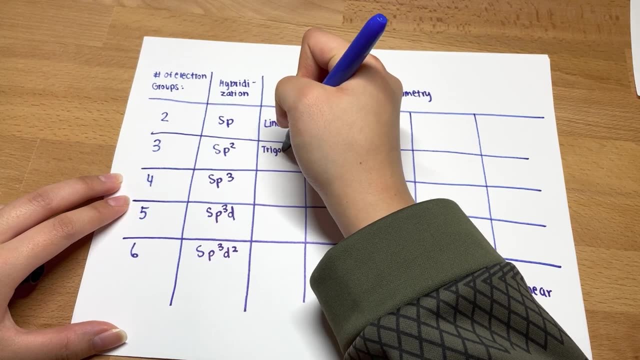 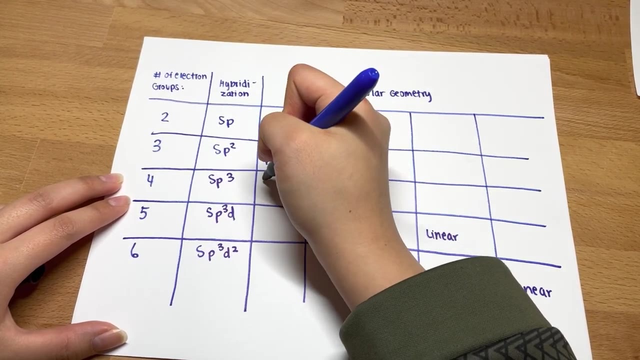 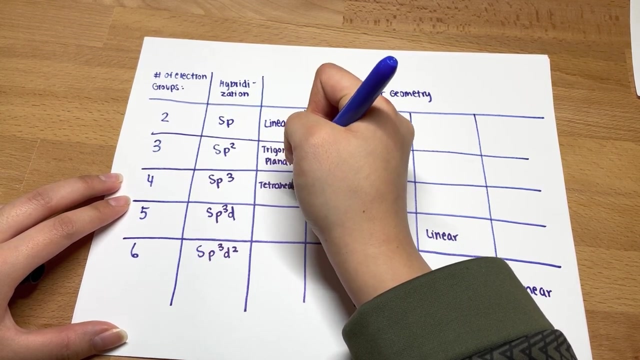 be fantastic. I feel like just remembering the electron group geometry is easy enough. so linear trigonal planar. imagine like three trigonal planar. now for the fourth one is tetrahedral. so think of Tetris. you know how. there's four blocks in Tetris, tetrahedral five. 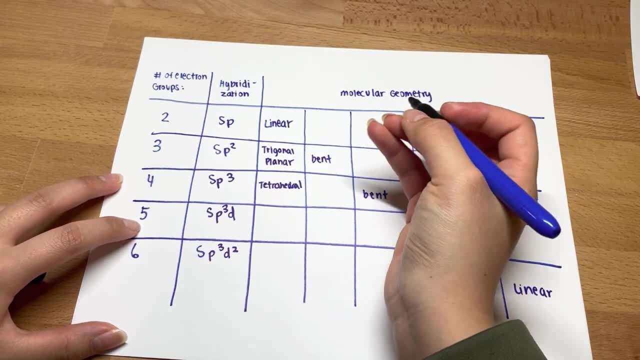 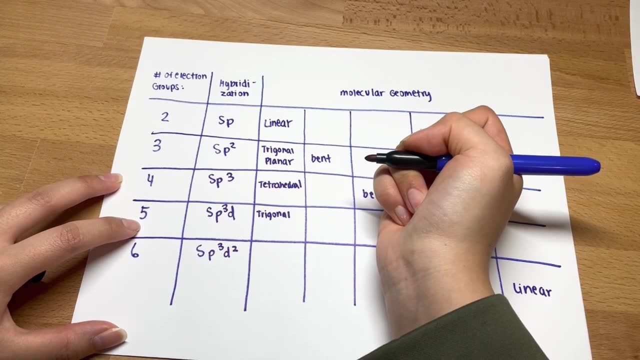 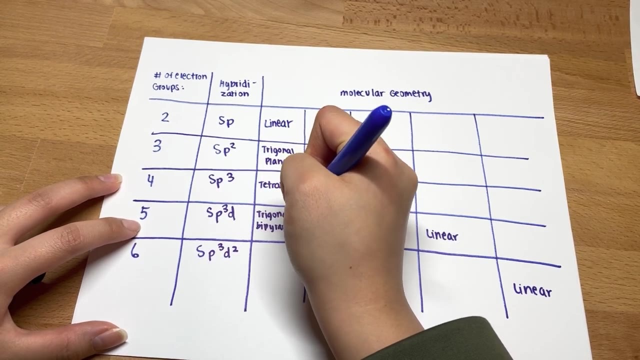 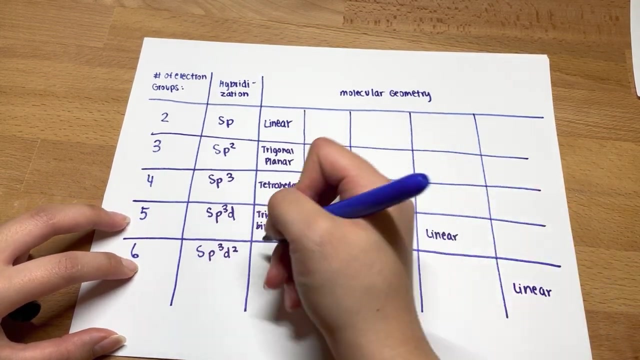 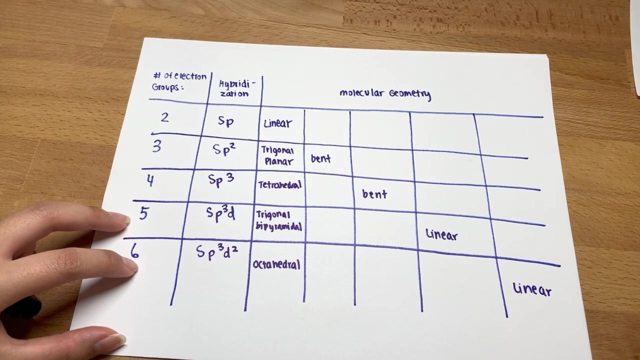 one is trigonal bipyramidal, so how I remember it. okay, so you do trigonal, which is three, right, by means two. so three plus two is five, so trigonal bipyramidal, this one is for the five and then for six octahedral. easy enough, right? okay, now you want to do. 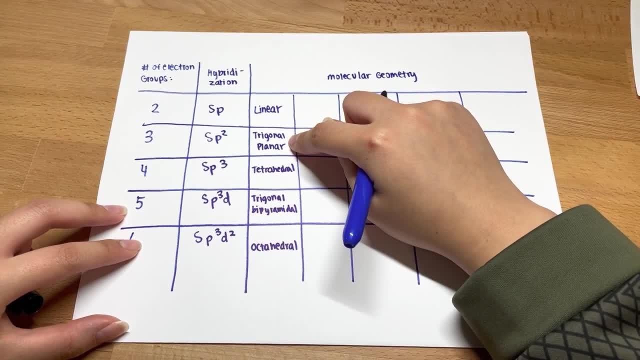 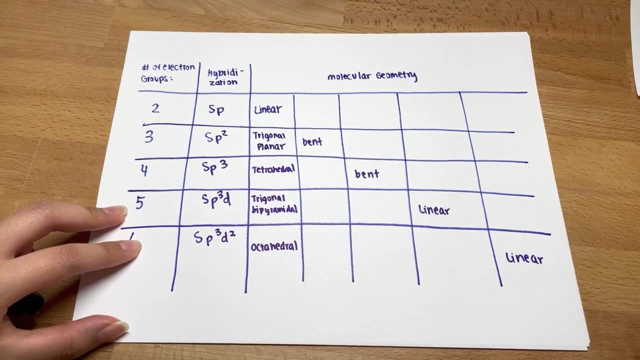 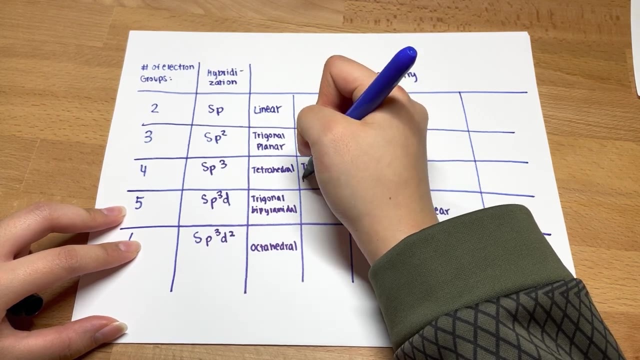 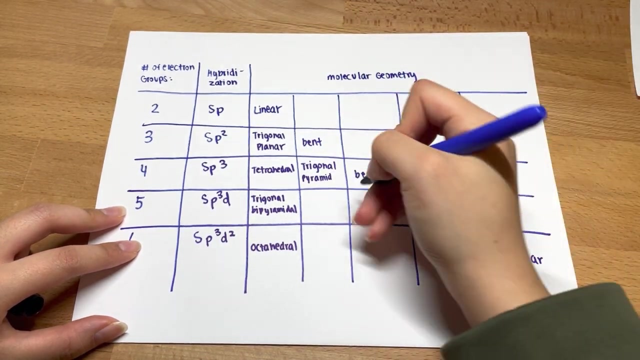 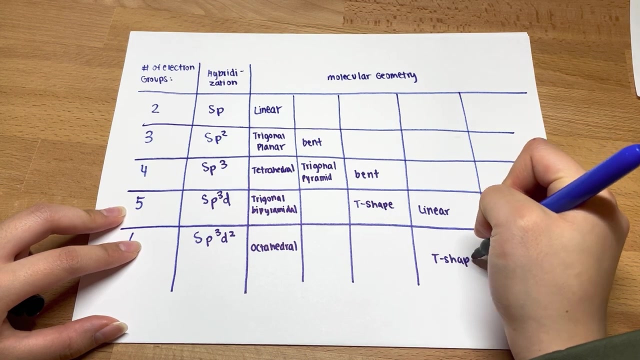 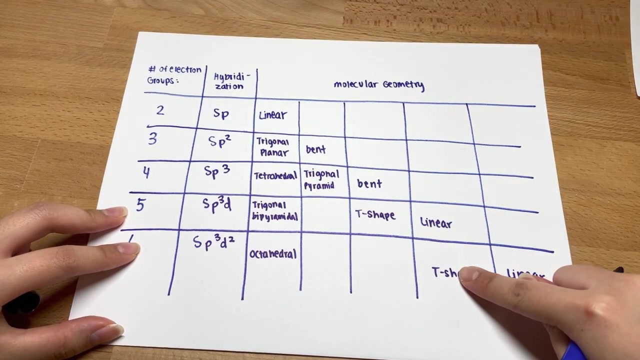 this, remember this trig plane trigonal trigonal planar trig mid t-shape, t-shape. so trig plane, trig mid tt. okay, trig plane trigonal pyramid, t-shape, t-shape. now let's review. so it will be linear, bent, bent, linear linear trig plane trig mid tt. you got the. 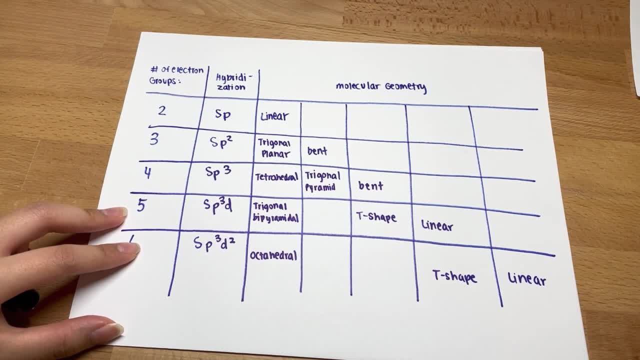 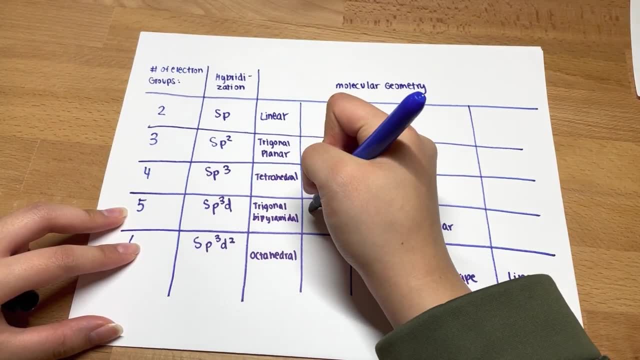 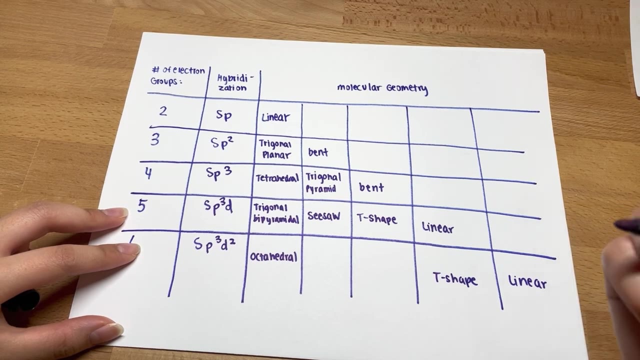 rhythm. okay, now this is the last one. this will be C, because you see this one before you can see this one, because this comes before this, so it'll be seesaw, and then we have only two left. we have the square pyramid and we have the square planar. 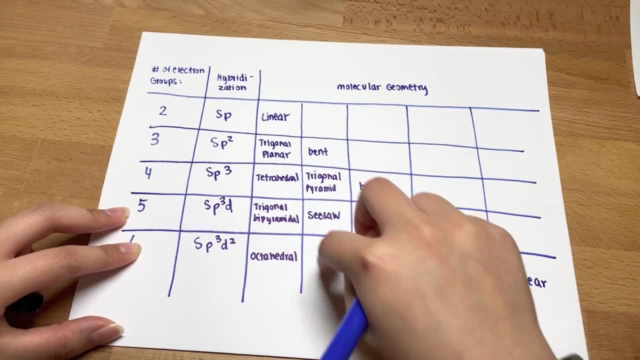 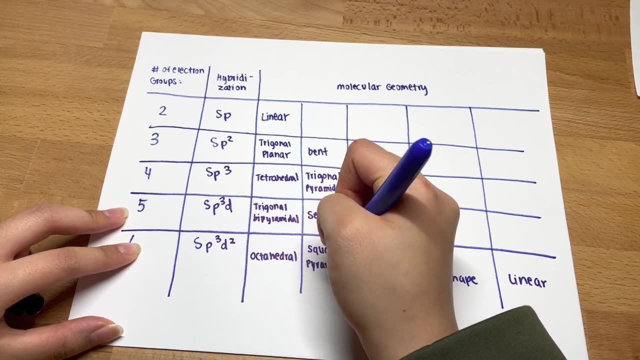 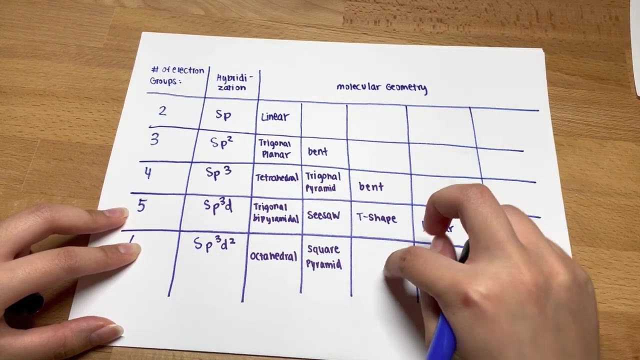 think of it like this: the pyramid will be with the pyramid, so the square pyramid will be here because it's close to this. so trigonal bipyramid and square pyramid close with each other. and then now we have only one, which is the square planar. so square planar. 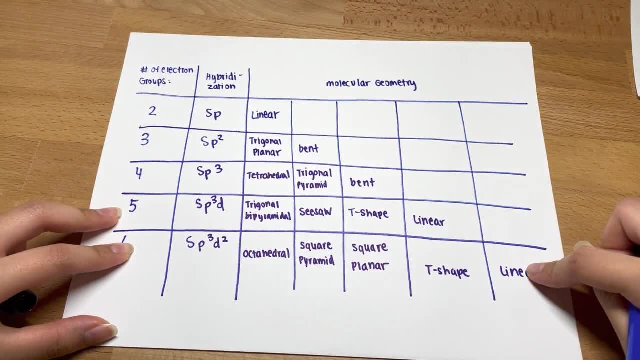 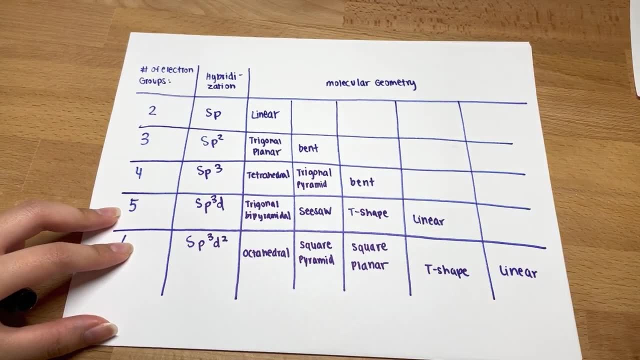 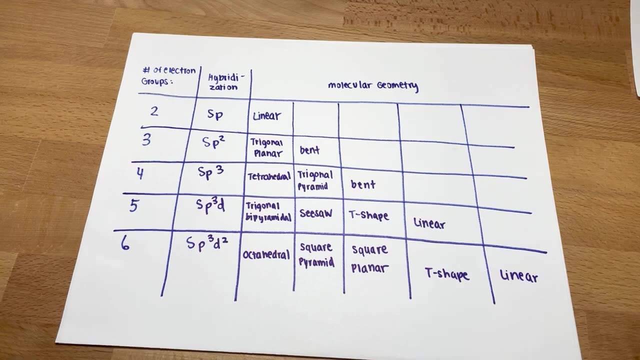 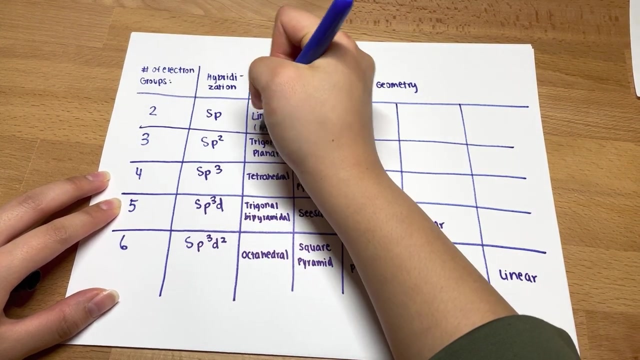 so let's review once again: linear bent, bent, linear, linear trig, plane trig, mid tt, c, square pyramid and square planar, and that's it. you remember? now I'm gonna teach you how to tell if it's polar or non-polar. this one is also easy. okay, it's just a pattern. this will be NP. this whole row will be NP. NP meaning non-polar, okay, 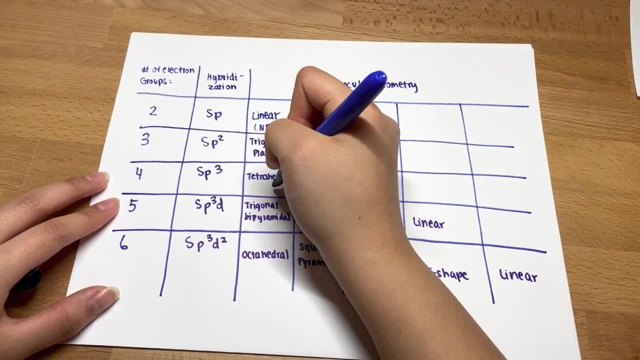 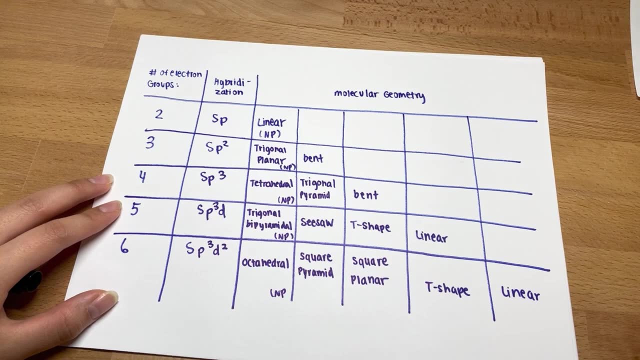 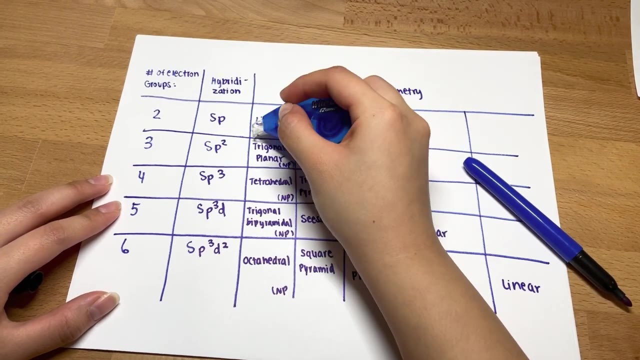 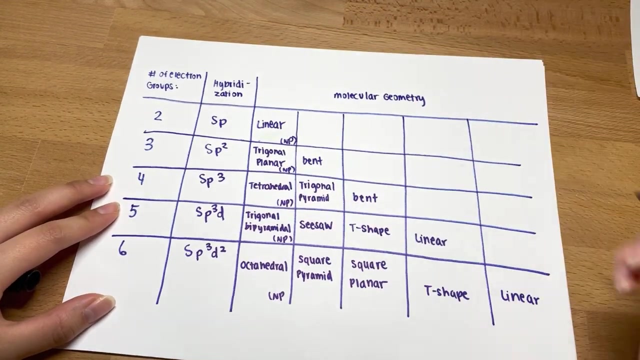 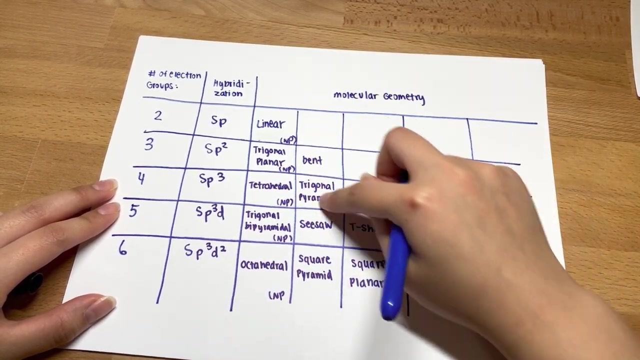 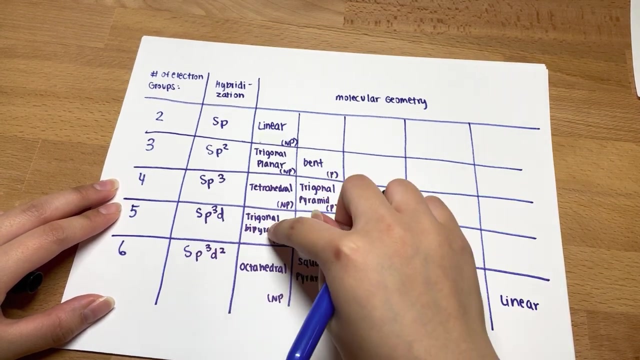 so write NP, NP, NP. okay, this one will be P, so it'll be like this: wait, let me write it so that it aligns together. it'll be like this: NP, NPP, NPPP. so all of this is P, all of these are polar, for this one is N, P, P, P, N, P. 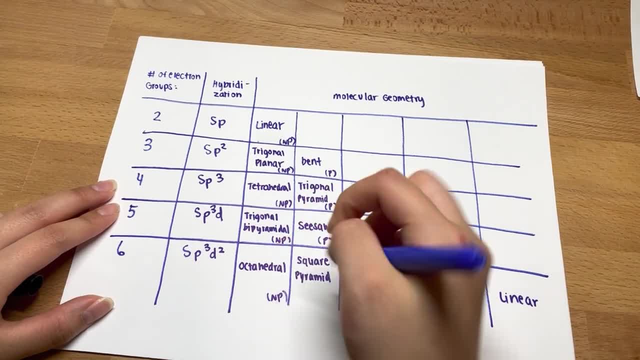 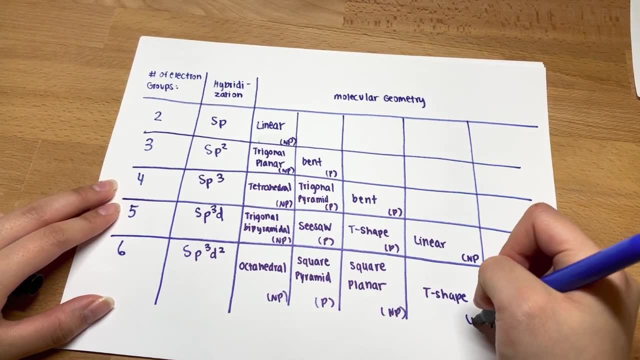 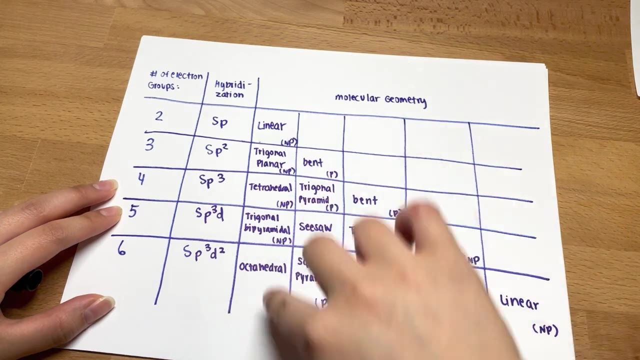 and for this one it's N P, P, N, P, P, N, P, N, P, P, N P. do you see the pattern? so all of these are NP. this one is N P P, this one, you just add. another: P N P, P P. this one, you add: 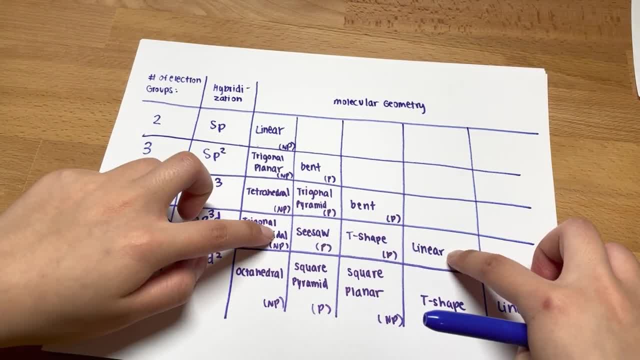 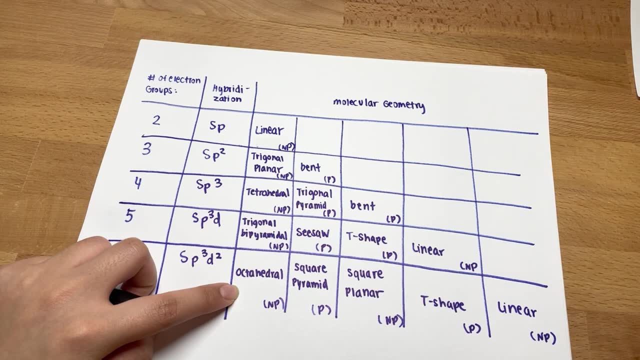 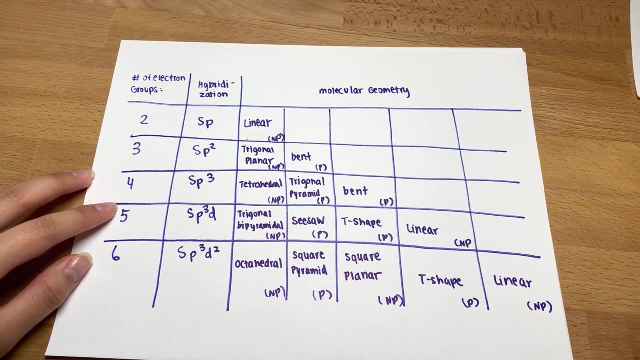 N, P at the end. so it will be like two NPs on the outside, two P's on the inside. this one you do NPP, NPP, NP. it's like a pattern: one, two, one, two, one, two and that's it. oh for the angle. if you want to know the angle this one is, since it's two, think of a. 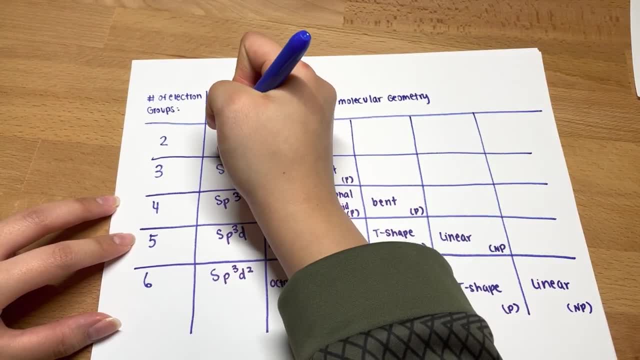 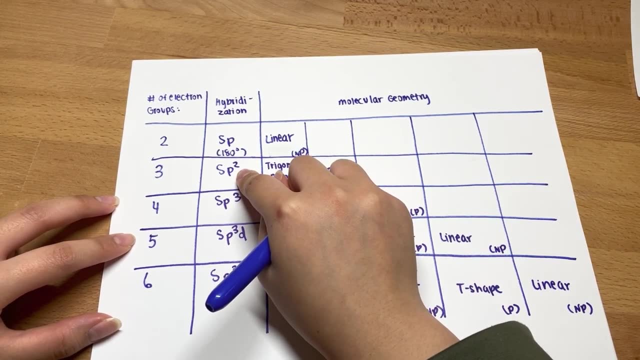 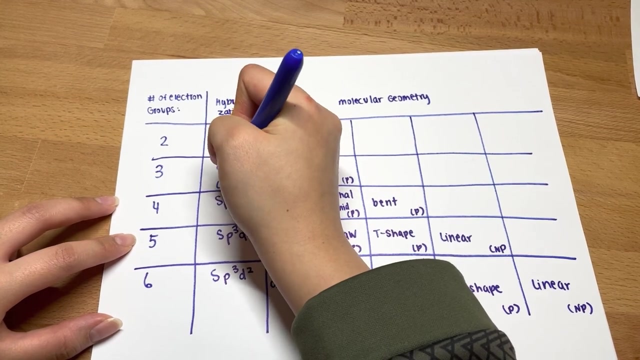 line, linear line. okay, the angle of a line is always 180, so 180.. for this one, since it's three, think of it as a triangle. so 120 times 3 is 360, right, so this would be 120 because you split it into three. and for four, 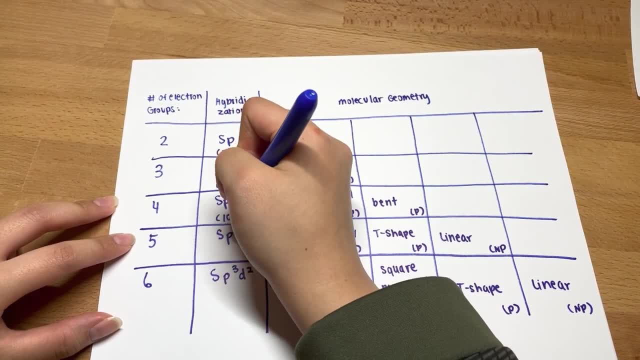 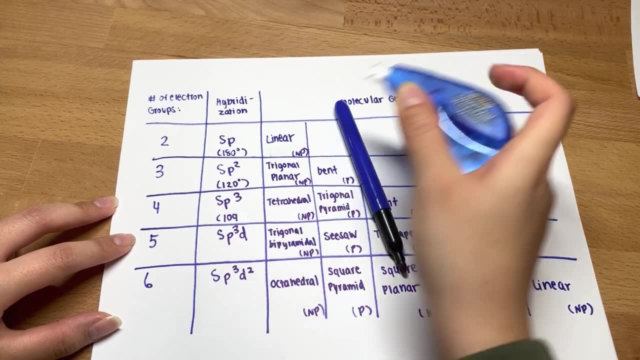 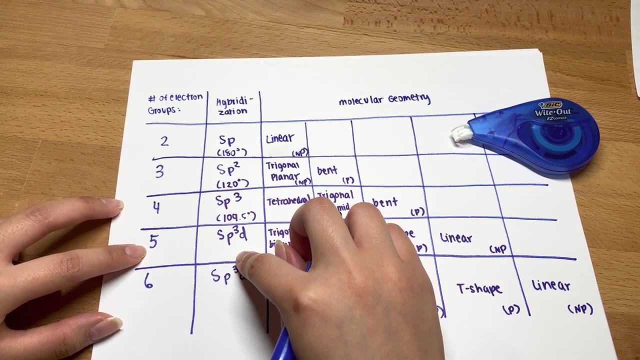 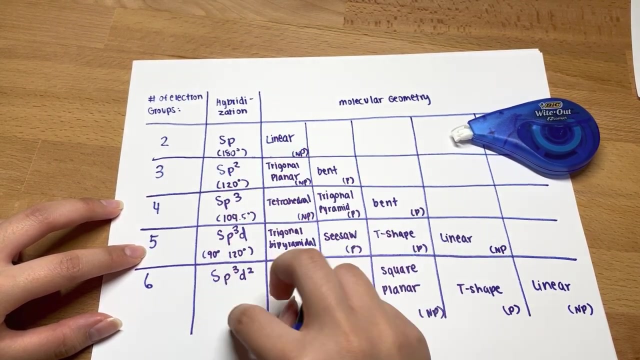 just remembered it as the only weird one. so it's like the 109.5 degrees, the 109.5, like this, and then for this one it's both 90 and 120, 90 and 120, and for this one it's 90- 90.. 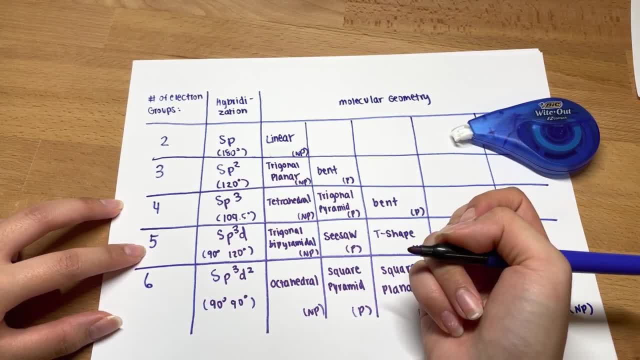 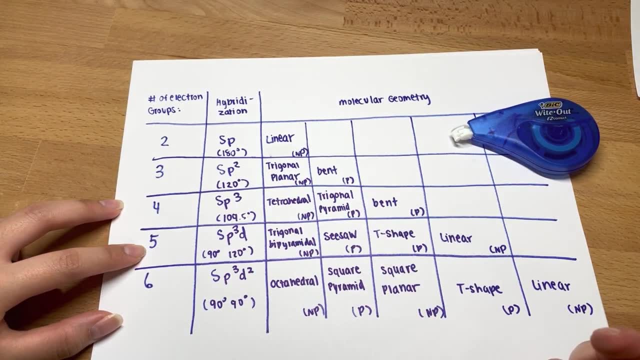 so yeah, 180, 120, 109.5, 90, 120, 90, 90.. that's it.